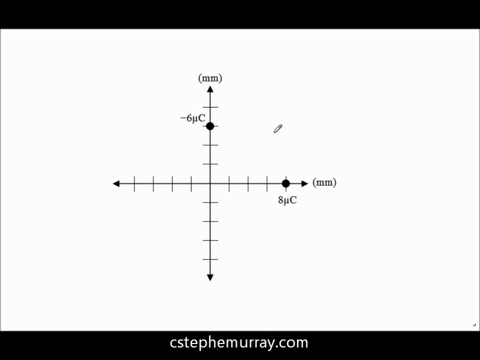 In this lecture I'm going to show you how to calculate the four basic electrostatic quantities, which are electric force, electric field, electric voltage- otherwise known as potential- and electric potential energy. First of all, notice our grid that we have. here We have negative six microcoulombs, which is negative. six microcoulombs is shorthand for times ten to the minus six coulombs, which is one millionth of a coulomb. 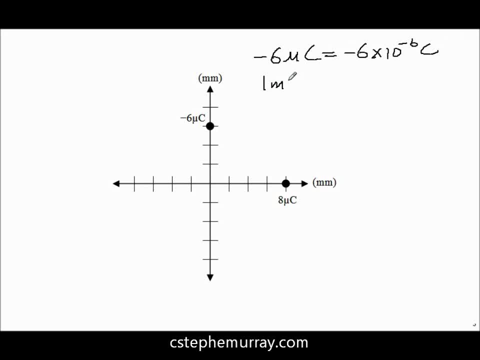 This millimeter thing. well, one millimeter equals .001 meter, or one times ten to the minus third meter. So again, when you see micro, you just put in your calculator times ten to the minus six. When you see milli, you put times ten to the minus three. 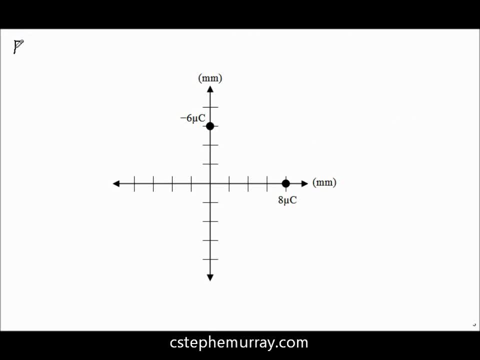 So the equations that we'll be using are: force, which equals k, which is nine times ten to the ninth absolute value, q1, q2, over r, squared, that's electric force. electric field, which is k, just one q. it only takes one charge to produce an electric field. 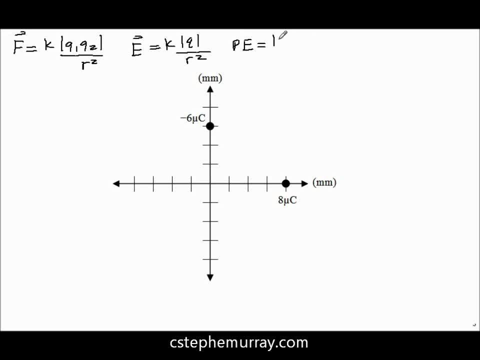 then potential, energy, which is k, q1,, q2, notice, no absolute values because it can be positive or negative, sorry, just r- and voltage, or electric potential, which is kq, again only one charge. So that's electric force which is necessary times r. 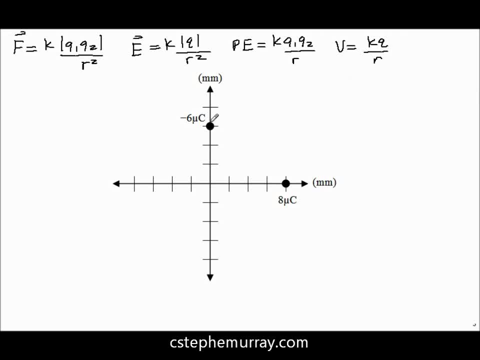 So those are our basic electrostatic quantities. Well, let's go ahead and start with electric field. You should notice that since this requires two charges and this requires two charges, we're going to calculate everything here at the origin and notice there's only one charge producing the electric field here. 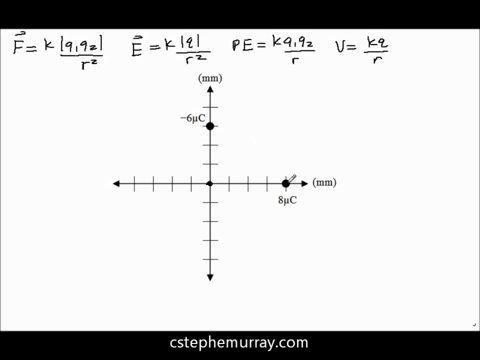 You may say: but look, there are two charges. We're not talking about the electric force here or the electric field here. The electric field is different everywhere. We're talking about at this point, at the origin. So at this point there are no two charges, there's only one. 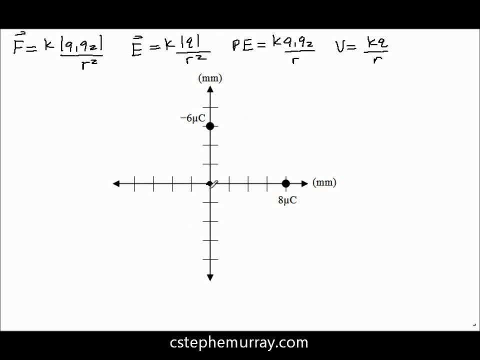 So electric force and potential energy are not valid. So let's find the electric field due to the minus six microcoulomb. Well, that's going to equal k. now this is the way I write it- kq now, it's absolute value. 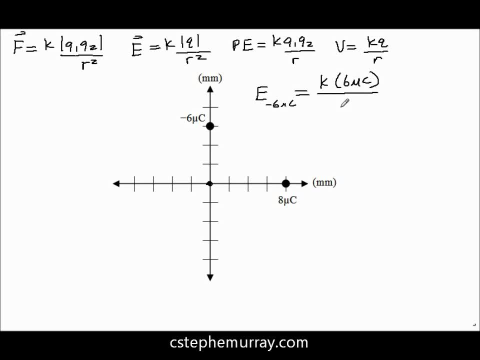 so I'm going to get rid of the negative sign r squared. these are millimeters one, two, three millimeters squared. but when I put this in my calculator I'm actually going to put in 99, six e minus six. 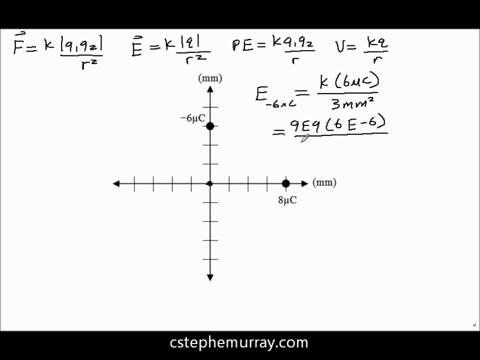 and twice. I'm going to do this. three e minus three, three e minus three. Now you should see Three times three is nine. so these are going to cancel Negative three. this is three, you know, ten to the minus one, six times, which is going to cancel out these. 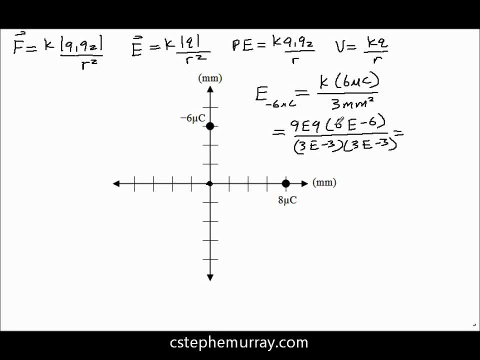 So the minus six and these cancel, and all I end up with is six times ten to the ninth, And that's newtons per coulomb, which, just so that we know for later on, is also volts per meter. All right, well, that tells you how to do this. 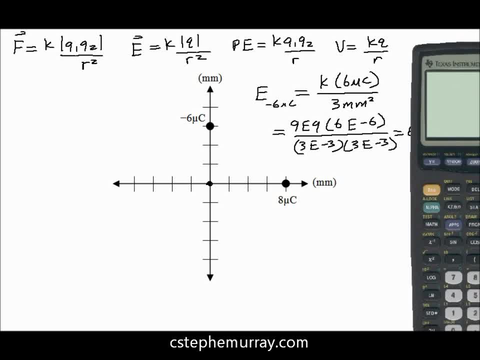 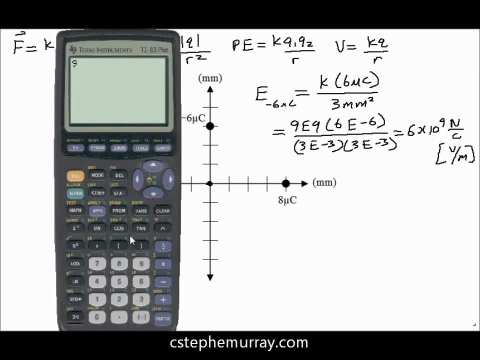 Now let's see if my, My online calculator actually works for this. so I'm going to pull this in and let's see if I can get this to work well. So if I were to put this in my calculator, I'd put nine e nine. you don't need to use parentheses because of that e. 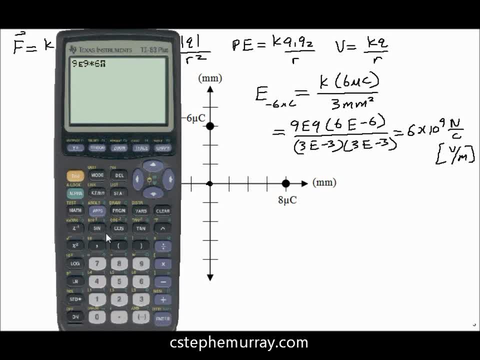 your calculator treats it just like a decimal: six e minus six divided by three e negative three, and I can just square that And there we go, exactly like we suspected. Okay, Move that out of our way. 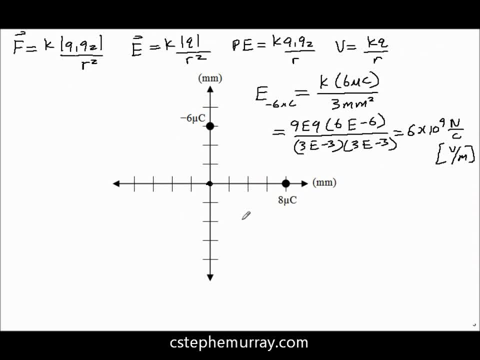 Our next one. we have this: eight microcoulombs, and our electric field here is e equals okay. well, let's just write it all out so that we can do the quick math. I tried to pick numbers so that we could do this easily. 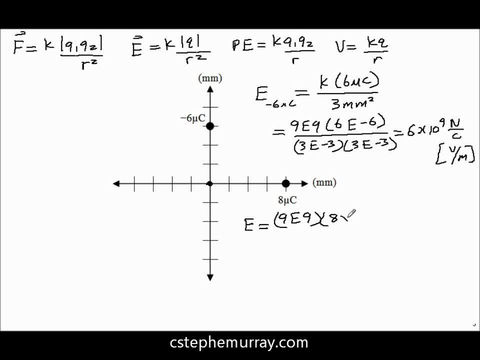 Ninety without the calculator. Eight ten to the minus six, And we have one, two, three, four And two of them. Again, the minus sixes cancels out. with these two, Eight comes into four. so how are we going to do that? 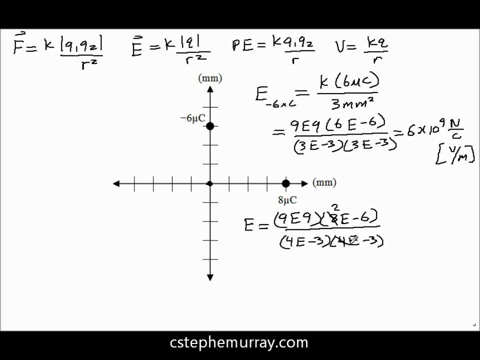 So this one would give us a two, so that one is gone And nine divided by four is 2.5.. Or I guess let's do this one, We'll take a two out here and we'll take a two out there. 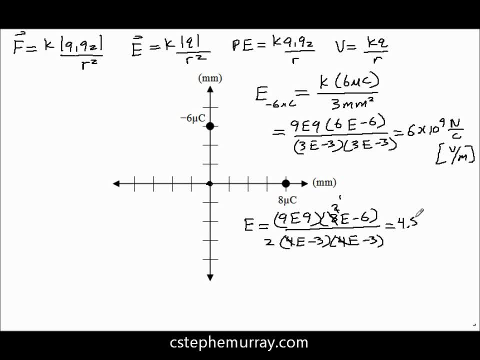 Two goes into nine, 4.5 times ten. to the ninth, units per coulomb or volts per meter. Now let's figure out the direction, What we do whenever we find direction. we always put a very, very small, positive test charge. 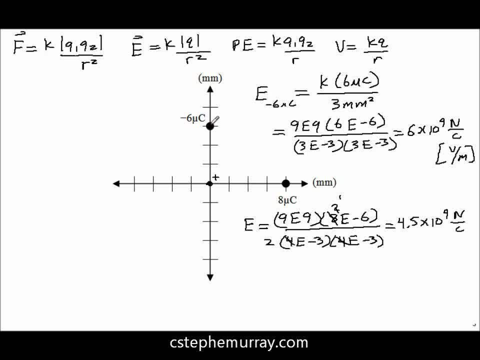 How small. Many students often say: well, if this is a positive, wouldn't it attract this one and push this one? Well, this is a positive. This is true, But we pick a very, very, very, very small positive test charge. 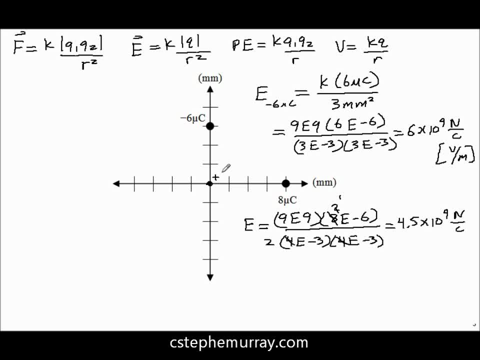 It's like, instead, you know, using something so small, the earth is not going to move when you drop a ball. So that's how small we're talking. This is so small that these are not going to move as a result, but we can use it to figure out the direction of the force. 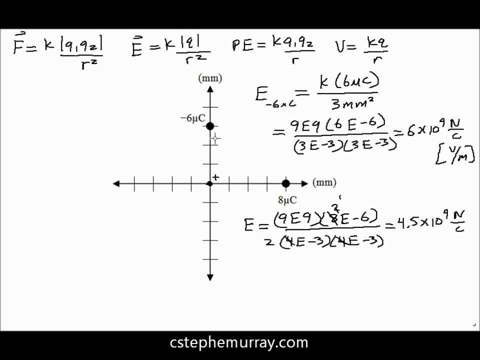 Well, this one is going to be pulled by it, So I'm going to put an arrow here. Doesn't really matter, I guess, which side. Okay, And unfortunately paint makes me have to do this the long way. There you go. 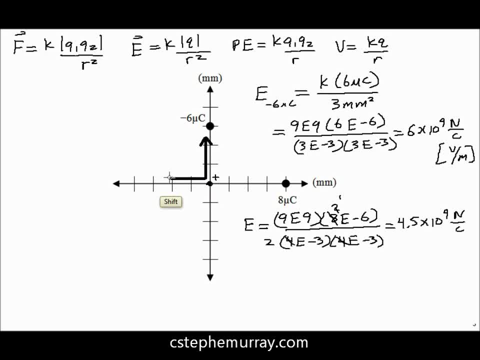 That's a pull And this one's a push because positive charges would push it. Now, the actual magnitude of these is different, but we're just going to show these And take this one, And actually you should be able to see that this is going to be pushed somewhere in the second quadrant. 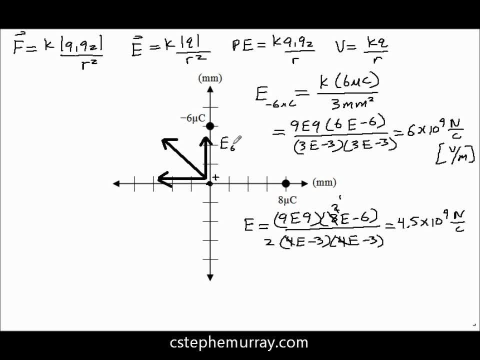 So this would be e due to the sixth. This is going to be e due to the eighth microcoulomb. This is going to be the net electric field in the second quadrant. So we now need to calculate what our net electric field is from what we had here. 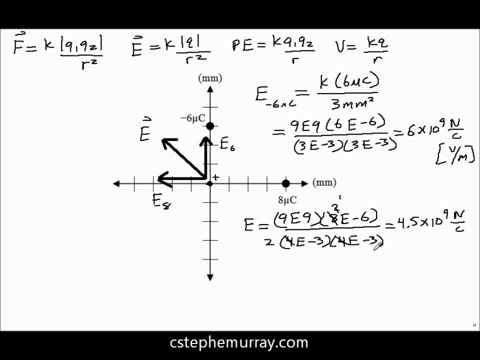 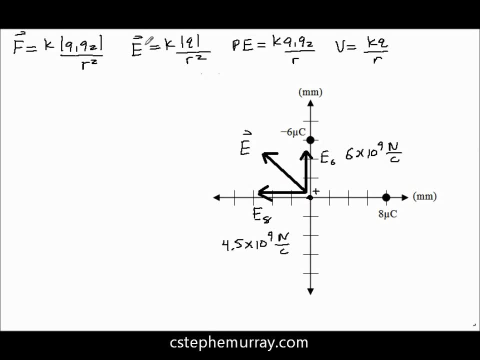 Let me go ahead and pause this, and I will go ahead and reset up the screen so that we can make this a little bit easier. All right, We've now moved things around so that we have a little less stuff on the page and we have plenty of room over here to work. 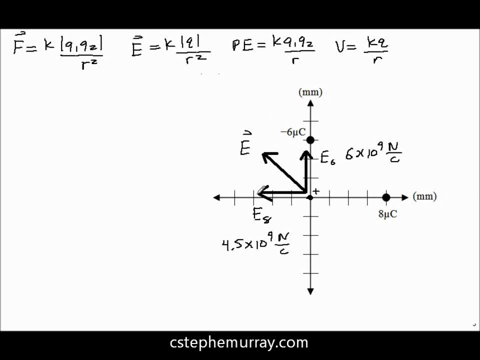 Remembering that electric field is a vector and we have two vector components that are perpendicular to one another. we know we must use Pythagorean theorem. So we know that our net electric field squared, our hypotenuse, must equal 6e9 squared plus 4.5e9 squared. 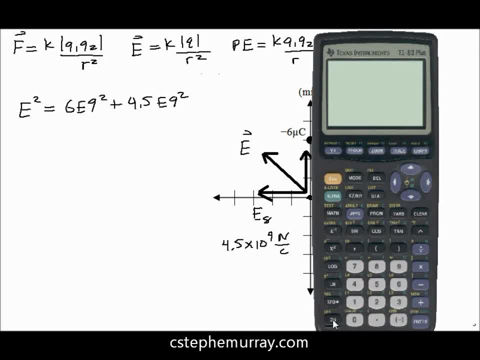 So let's go ahead and bring in our calculator over here. Let's hope we're working easily here. Good, e9 squared Plus 4.5e9 squared equals. take the square root, the answer. you don't even need that 7.5.. 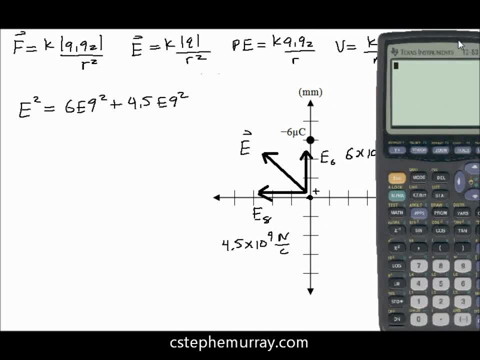 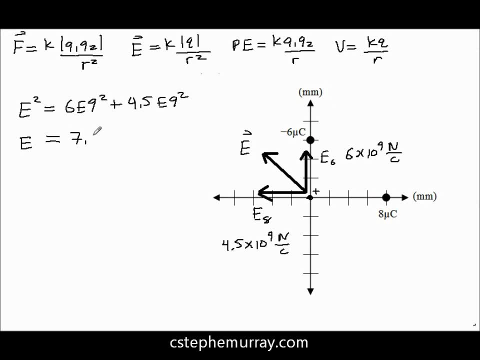 Thank you, We'll clear that and come back and use you later. Equals 7.5 times 10 to the ninth Newtons per coulomb. So what about the direction? Well, we generally take all of our directions here from the x-axis. 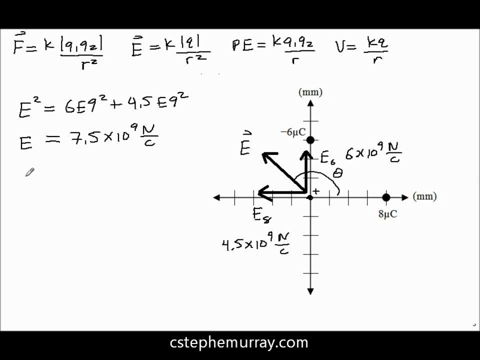 Now you could find this one right here, which would be just fine. And when we do ours from the x-axis, we say the tangent of the angle equals the opposite, which is generally y over x, Or that theta equals the inverse tangent of y. 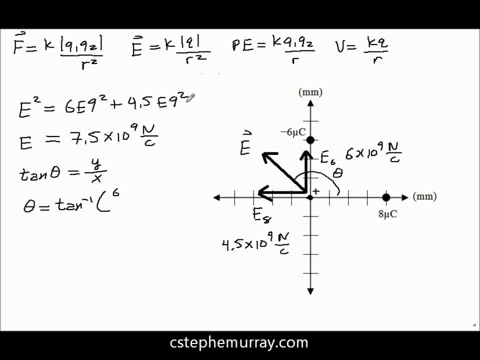 Which is a positive 6.. Now notice these 9s all cancelled out. I'm going to write this just so that you understand why we don't really have to write all this. I wouldn't be writing this except that I'm showing you guys this. 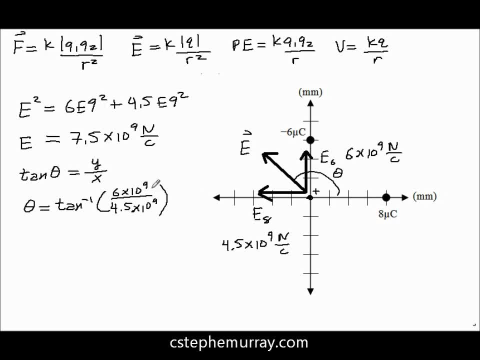 You see how there's a 10 to the ninth on the top and a 10 to the ninth on the bottom, So all you really had to do was the inverse tangent of 6 over, and actually that's pointing to the left, which is a negative 4.5.. 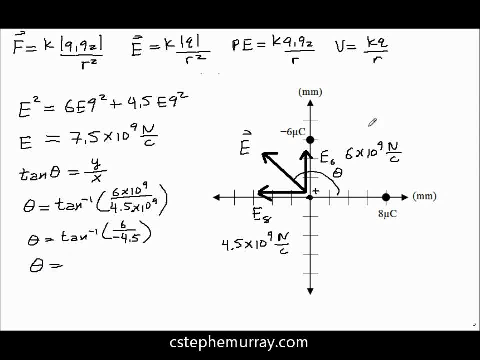 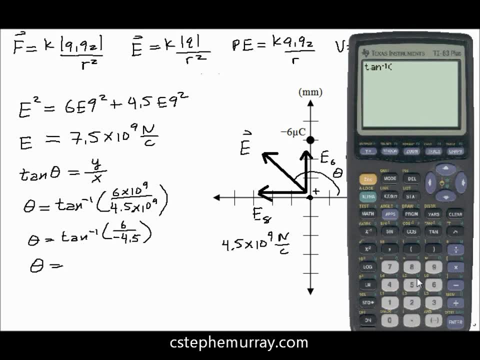 Well, theta equals 4.5.. Well, theta equals- let's bring out ti again. there it is. So we'll take the inverse tangent of 6 divided by negative 4.5.. And that gives me that's: oh darn, we're in radians.